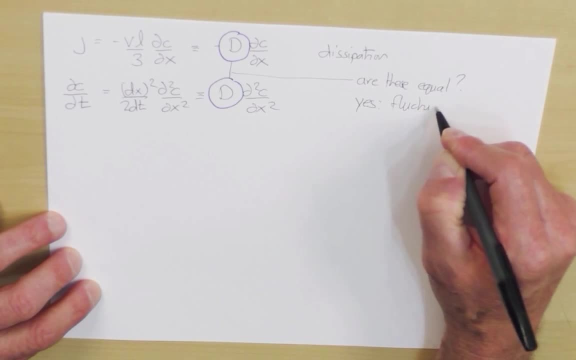 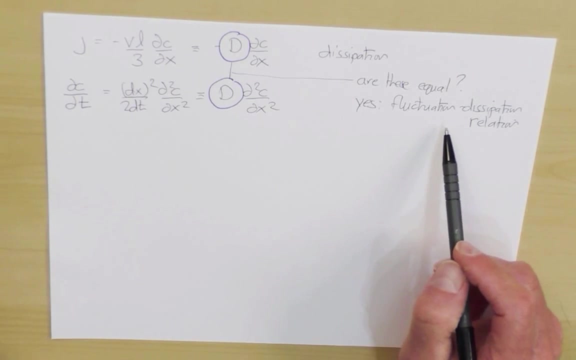 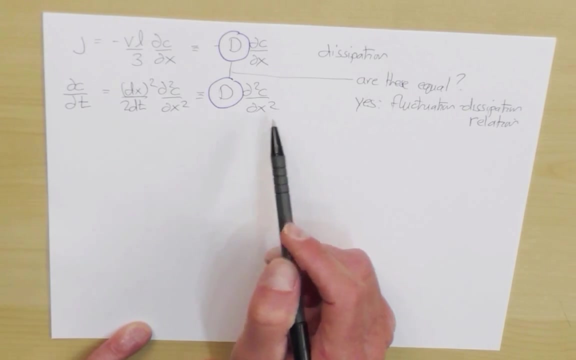 actually a manifestation of something called the fluctuation-dissipation relation, Because it relates- something that describes the dissipation of a concentration gradient, to the random fluctuating motion of a random walk. So this line could be viewed as a fluctuation quantity, And so the point is that there is a deep relation between dissipation and fluctuation. that's embodied. 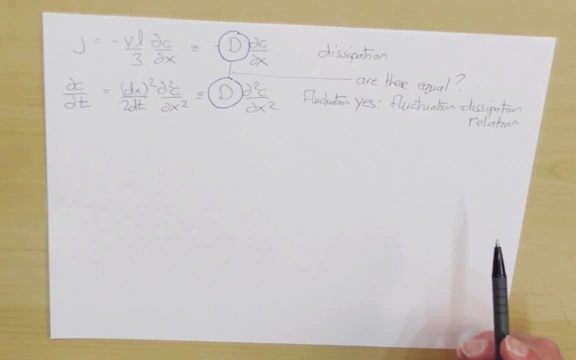 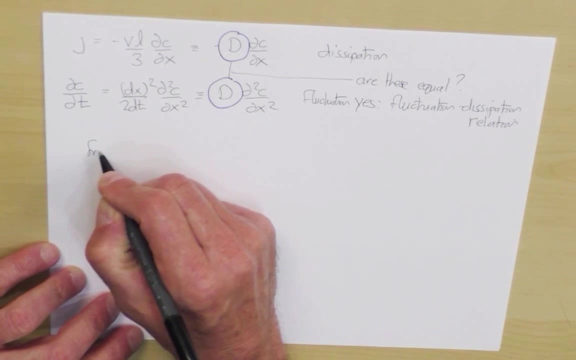 by the fluctuation-dissipation relation. Now I can't show this in general, but I can kind of wave my hands and give you a feeling for why this ought to occur. So let me just remind you from earlier in the lectures that from kinetic 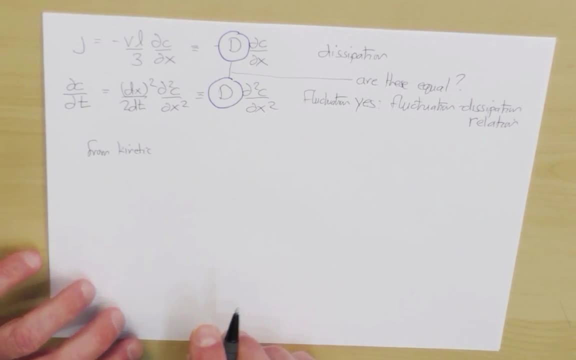 theory of gases and basically kinetic theory is just a simple picture in which you think of a gas of particles, like the gas in this room. It's basically made out of billiard balls And these billiard balls are just zooming around at roughly 300 meters per second And whenever they collide, they collide. 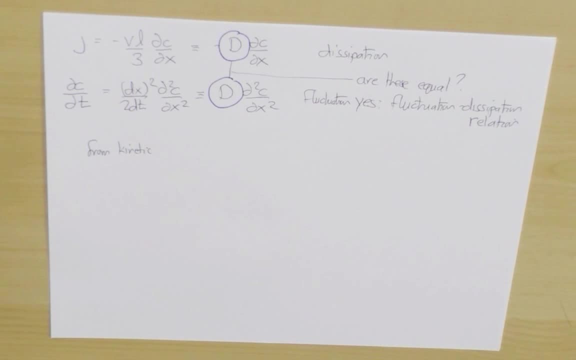 elastically, And so there's a lot of randomization of the motion of the particles because of these relatively frequent fluctuations. And it's thermal energy from the outside that's providing the energy that propels the molecules, But once they're moving at 300 meters a second, they more or less move at that speed. So in this kind of a picture of 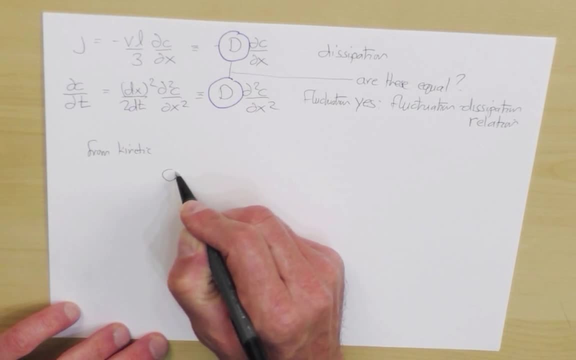 molecules or billiard balls bouncing around if we follow just a single billiard ball. so here it is and it moves until it collides with another molecule and then it gets scattered in some arbitrary direction. Now this molecule has a cross-sectional area sigma. 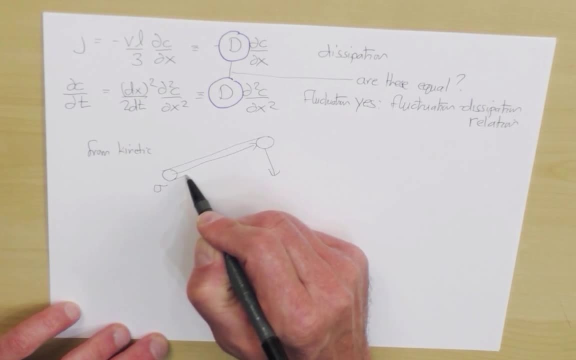 So, as it's moving about, it sweeps out a collision tube whose radius is roughly of the order of the square root of the cross-sectional area of the molecule, And it goes a distance L, And we determine the characteristic distance that a particle moves before it collides, the mean free path by the criterion that when there is of the order of one other. 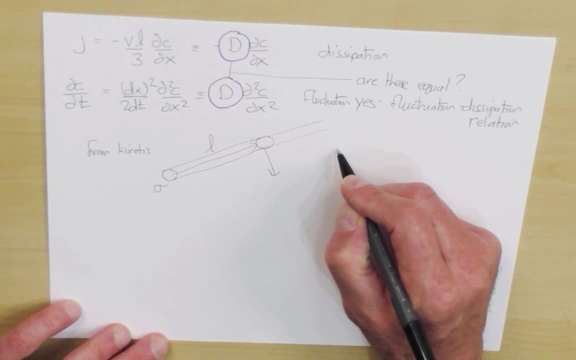 molecule in this swept out tube, this collision tube. so the volume of the collision tube is the length of the tube times the cross-sectional area of the tube. The number of molecules in the tube will then be the volume of the tube times the concentration, When this is of the order of one, that defines the collision. And so we infer from this that the mean free path the 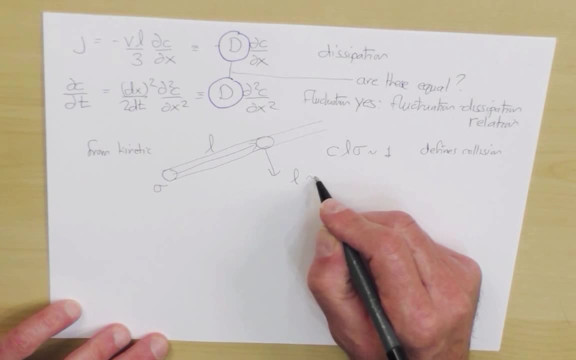 typical distance a molecule moves before it collides with anybody is of the order of 1 over C sigma. And as a matter of interest, just to get a feeling for numbers, the concentration of a gas, say, in this room that's found by the 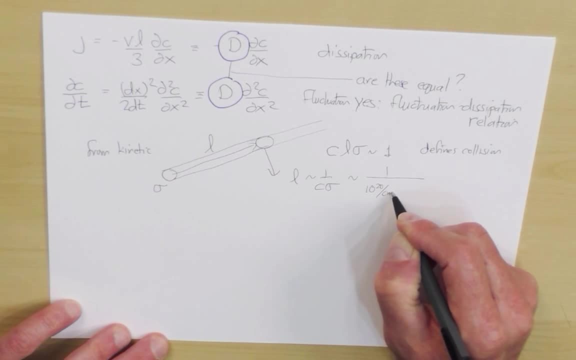 is 10 to the 20th molecules per cubic centimeter, and the typical diameter of a molecule is of the order of a couple of angstroms, and so the cross-sectional area is a couple of angstroms all squared, which is roughly 10 to the minus. 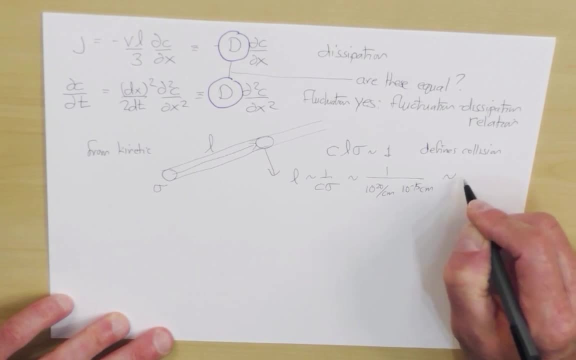 15th centimeters. So the mean free path is some number of the order of 10 to the minus 5 centimeters, which is of the order of a hundred to a thousand molecular diameters. So this gives you a feeling, for, like the nature of the 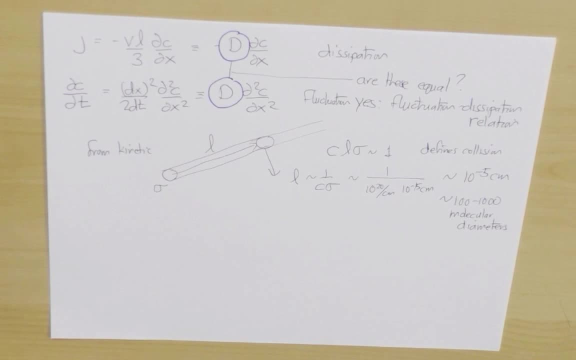 motion of molecules in this room. They're all moving roughly a thousand of their own diameters before they bump into somebody else. And we can also ask what is the time between collisions? And the time between collisions is roughly the distance that the molecules go between collisions, divided by the thermal. 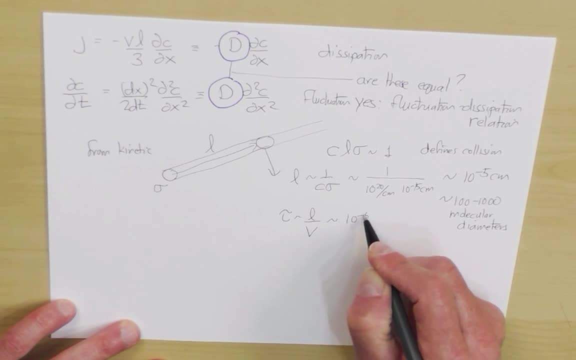 velocity, And this 10 to the minus 5 centimeters. the typical thermal velocity is 300 meters per second roughly, or that's 30,000 centimeters per second, and so this collision time is of the order of 10 to the minus 9 to 10 to the minus 10. 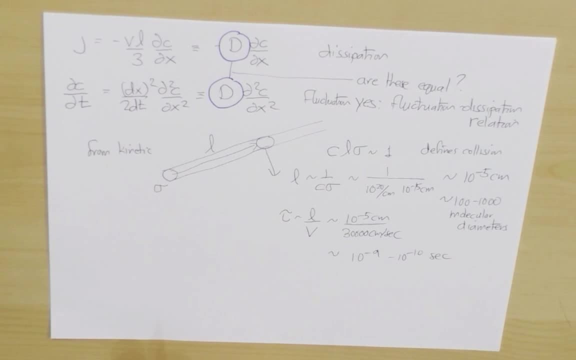 seconds, so roughly a billion to 10 billion times a second a molecule experience. a molecule experience is roughly a billion to 10 billion collisions per second, so it's pretty impressive. so finally, to motivate or to attempt to argue for this, dissipation of fluctuation: dissipation relation.